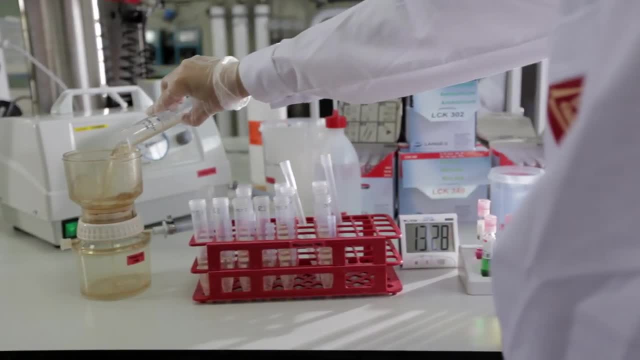 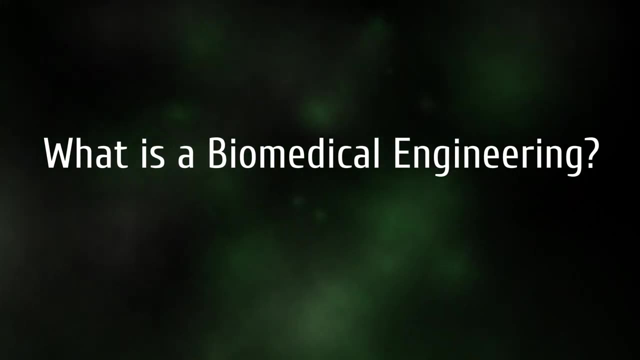 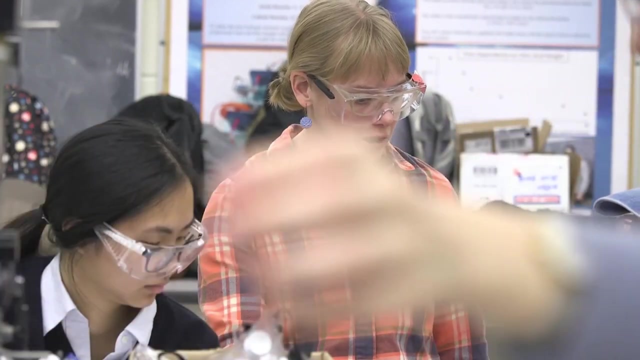 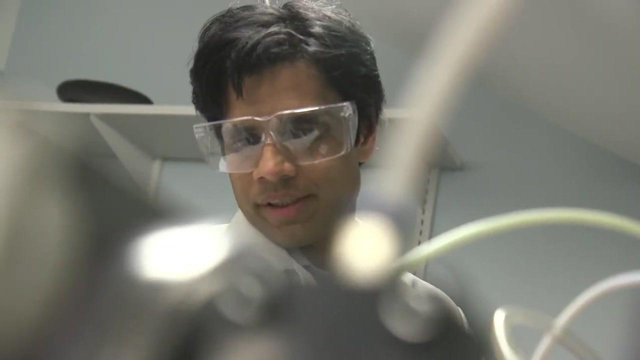 I hope now you are ready to know about biomedical engineering after the career selection topic. What is biomedical engineering? Biomedical engineering, or BME, is the application of engineering principles and methods to solve medical and biological problems. It also integrates electrical, mechanical, chemical and life science principles in the development of new 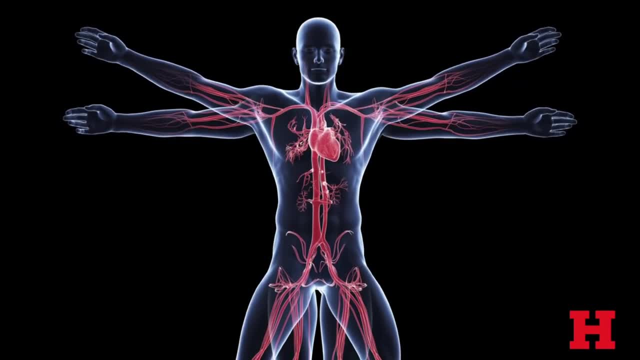 healthcare technologies and systems. This was the definition, But if I had to name a specific model, I would name it BME or BME-BSTAR. Now, if I were to explain the term biomedical engineering in a simplified way, it is how: 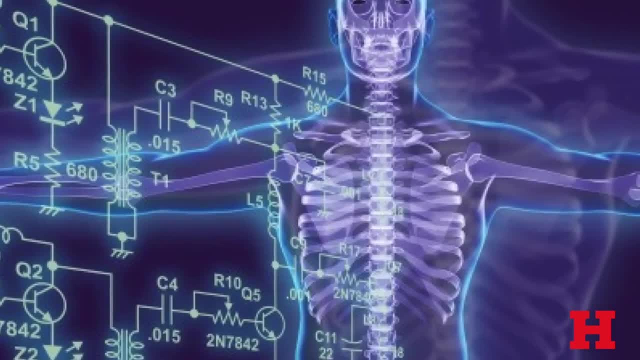 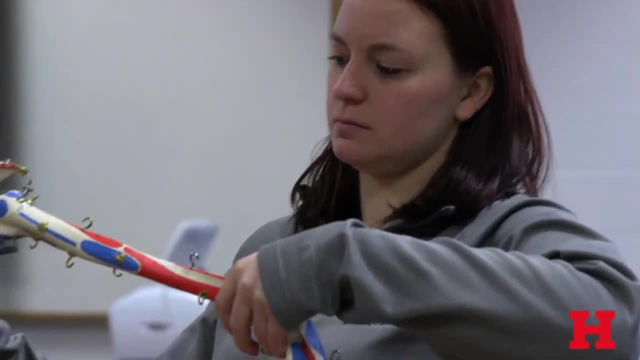 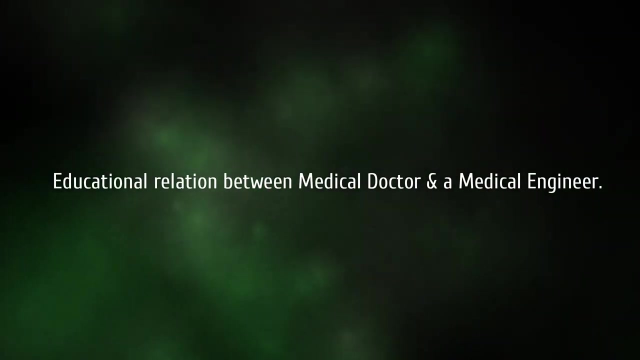 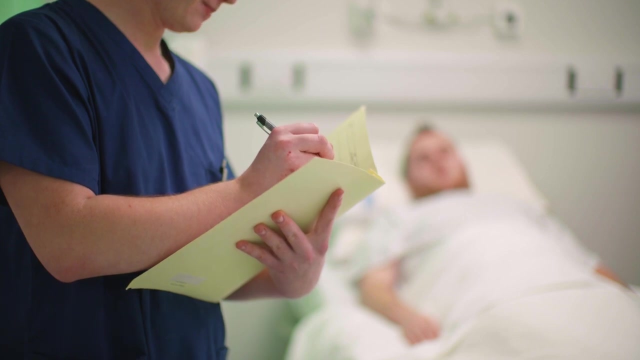 you develop an external body organ to support an internal body organ or developing a diagnostic device or monitoring device to support the medical condition is called biomedical or medical engineering. Educational relation between medical doctor and a medical engineer System. work is somewhat same. doctors complete MBBS and chose specialization which they 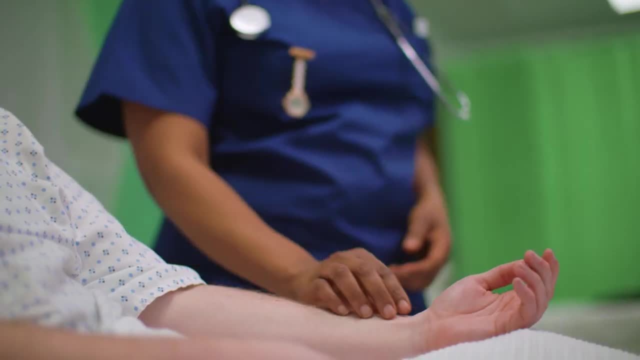 like to work on, like urology and chemistry. Classified medical engineering is a type of medical engineering where doctor and medical engineer work mixed in a mäu–psi or네 decision. cardiologists take care of kidneys, cardiologists take care of the heart and so on. 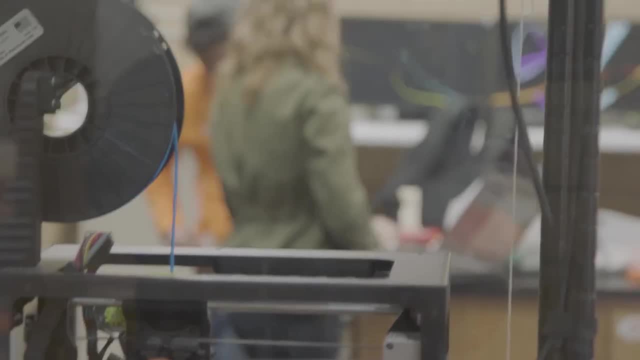 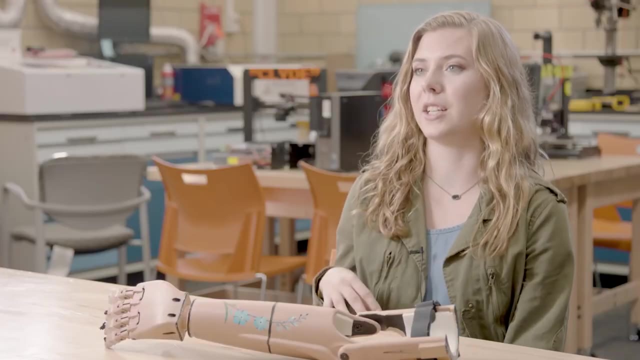 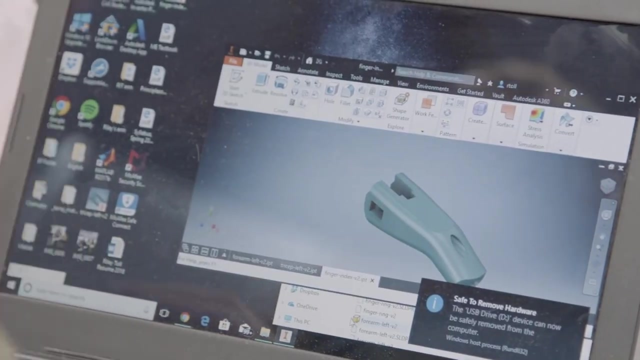 In the same manner, you can complete biomedical engineering and can be specialized in specific equipment like EEG, ultrasound, MRI, x-rays and any number of equipment which is used in the healthcare sector. It is very crucial to know which sector you like to work after completion of your diploma. 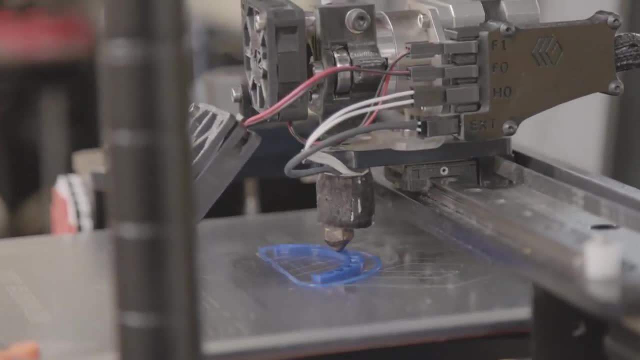 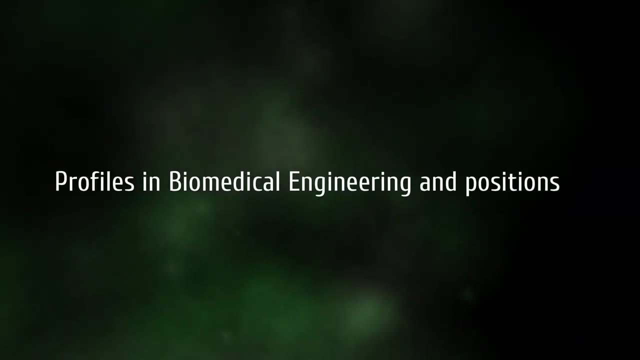 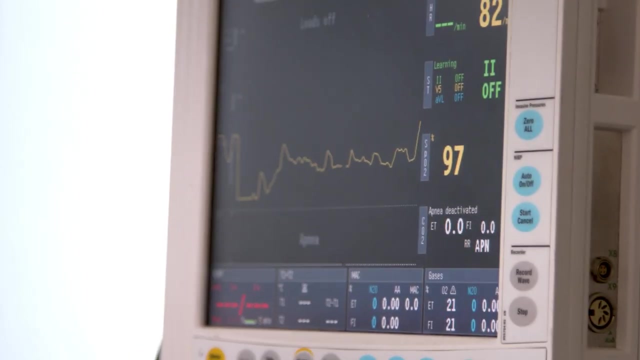 or bachelor program. If you like to research and want to invent a new medical device concept, then you can work with many research companies in the health sector. Job Profiles in Biomedical Engineering and Positions. When the word engineering involved in any field, it is related to know the answers. 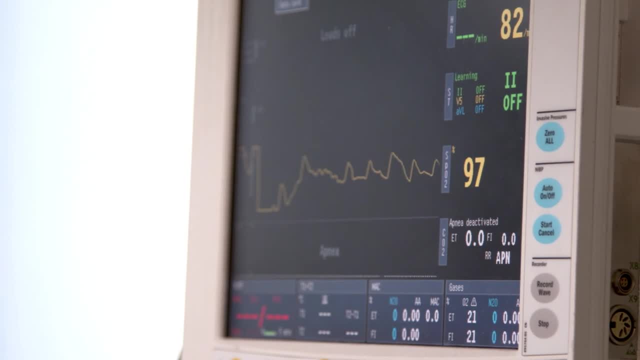 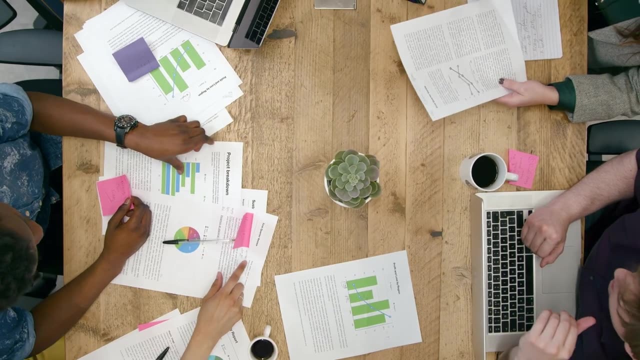 technicalities and come with ideas to resolve the needs. Same way, in biomedical engineering stream, you will be learning about existing technologies available in the medical sector and getting into the research to develop the same product or a new product which will be in compliance of medical grades. 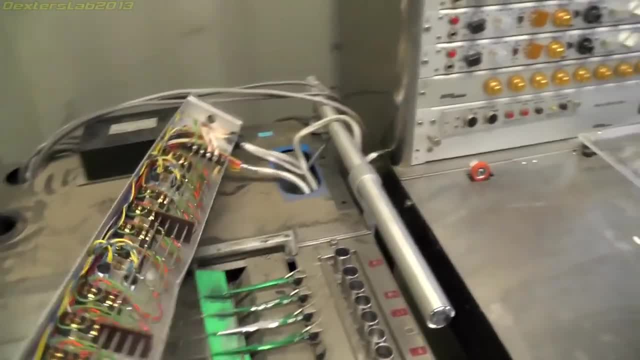 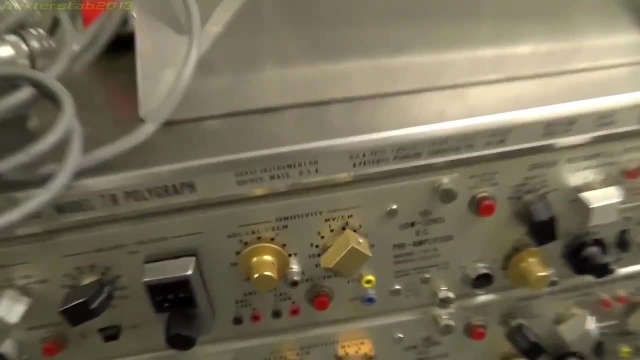 As an example, in 1935, Albert Grass first built his three-channel EEG machine, which works on battery, at the Harvard Medical School, and as technology advanced, he, with his wife Ellen Robinson Grass, formed the Grass Instrument Company in 1945.. 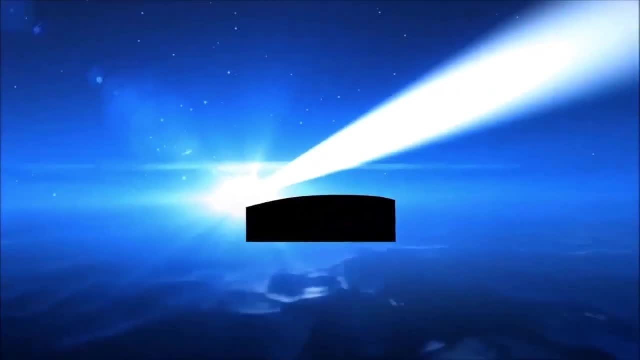 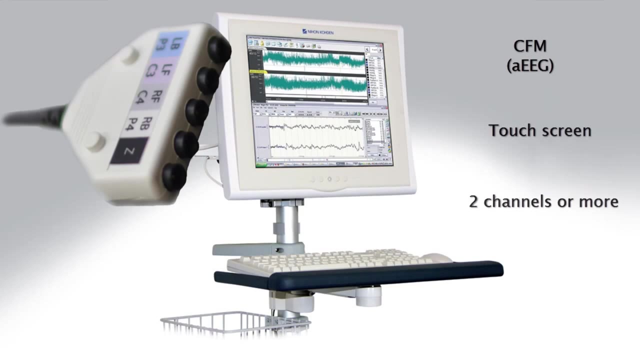 In the same manner, Nihon Kodan has invented, successfully developed the ME-1D, the world's first eight-channel direct-writing EEG that was completely AC-powered in the 1950s. So if you are more interested in learning more about the EEG, please subscribe to our 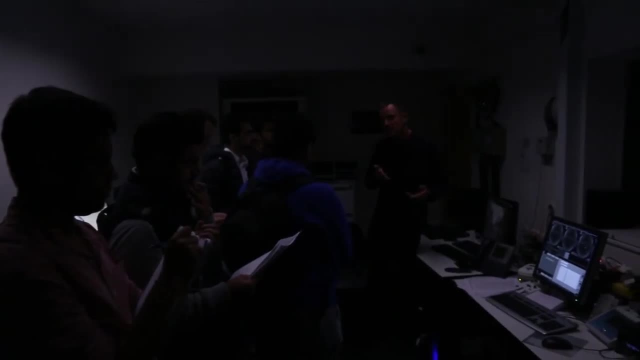 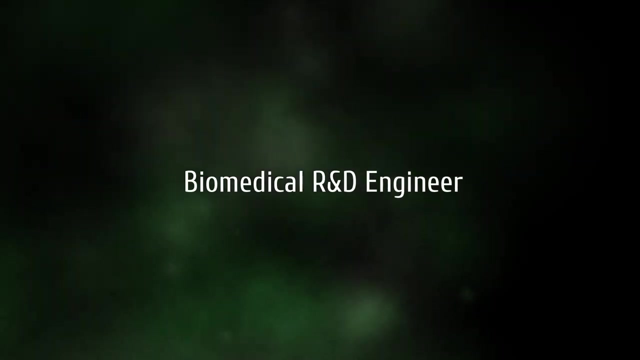 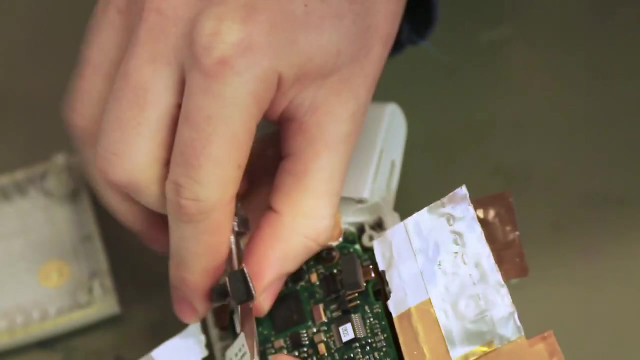 YouTube channel. The first professional profession once you complete biomedical engineering can be R&D engineer, but this type of job mostly given preference to the students who have been completely into research throughout the academics while pursuing biomedical engineering. The second profession is sales and marketing engineers. 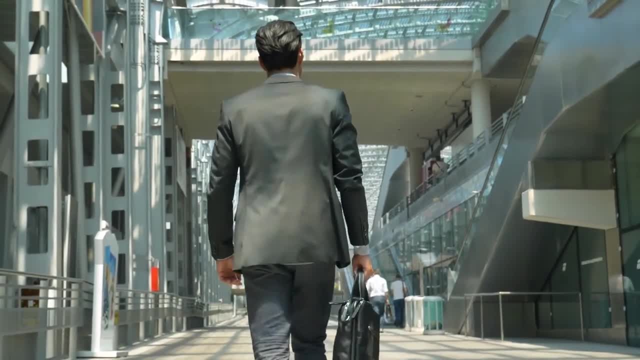 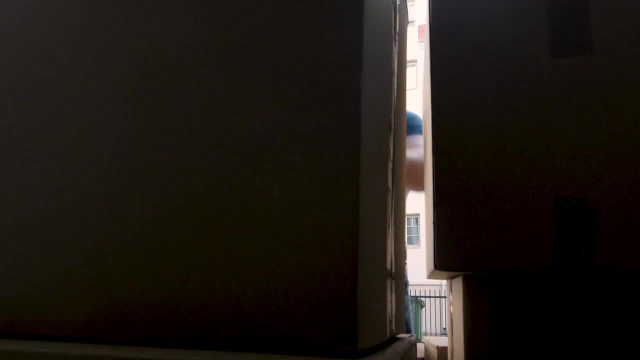 If you have pursued the MBA marketing program after biomedical engineering and if you have a good sales marketing skill, Then there are many companies where you can work on different positions in the company for sales and marketing of a medical product. The third position is application specialist. 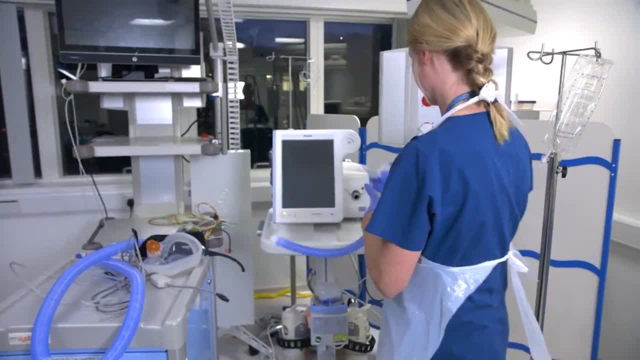 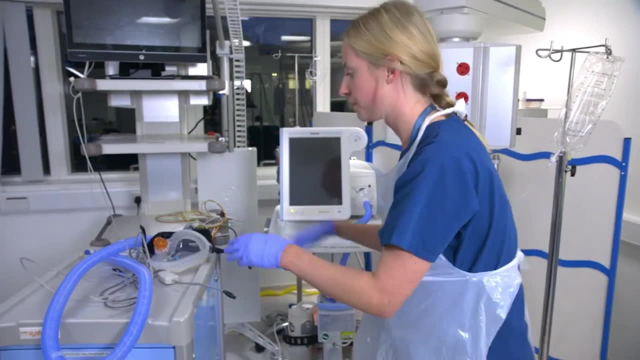 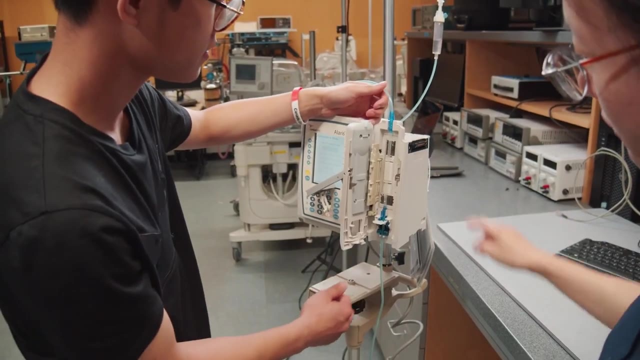 This is also known as pre-sales and post-sale application specialist. Their role is to educate the users in a hospital. This is also a part of sales and marketing. If you have very good communication skills and interaction with the doctor, then it's one of the most learning and challenging roles in biomedical industry. 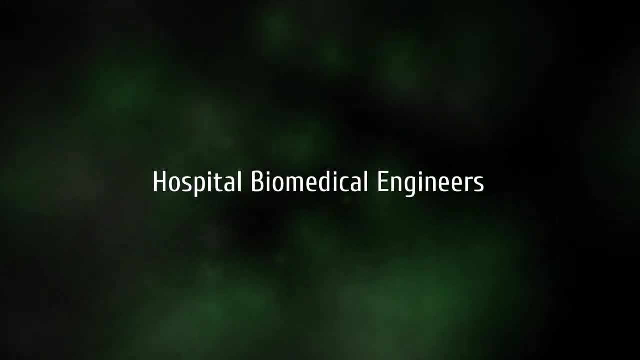 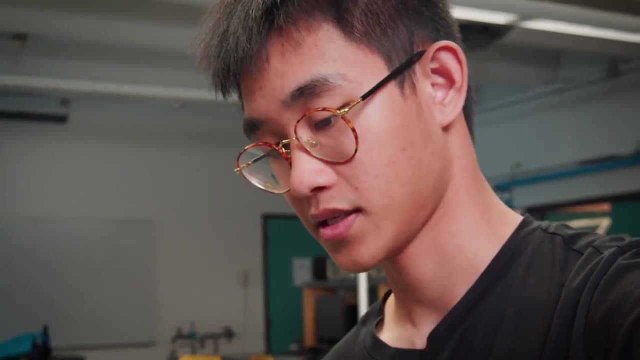 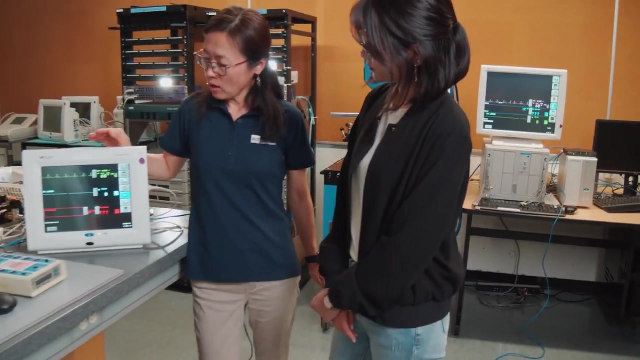 The fourth position is application specialist. The fourth job position is hospital biomedical engineers. This position plays a vital role in the hospital. In this profile you need to maintain all records of the medical equipment's decision need to be made for purchasing a medical equipment in hospital, reducing breakdown time of medical 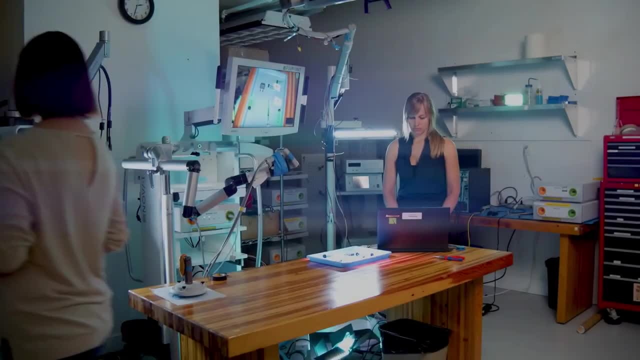 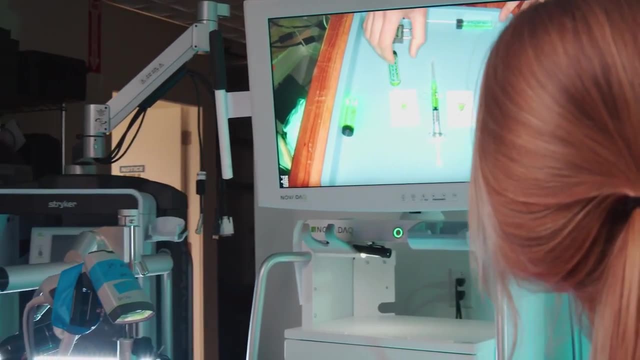 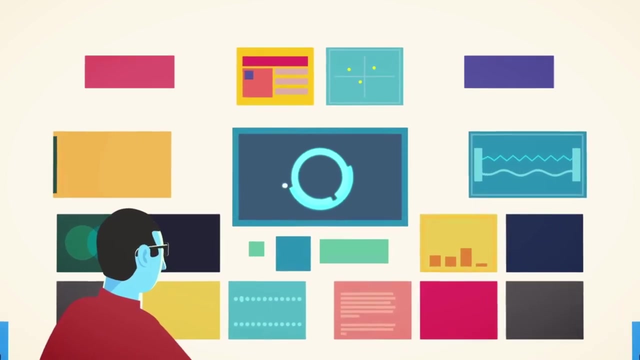 equipment. annual calibration and preventative maintenance of all medical equipment, Educating users about how to use the medical device, cleaning process and maintaining the life of medical reusable accessories. These are the very few points in which this role in biomedical engineers perform in hospitals. 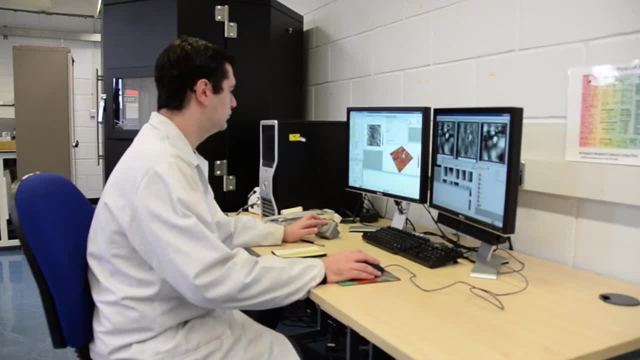 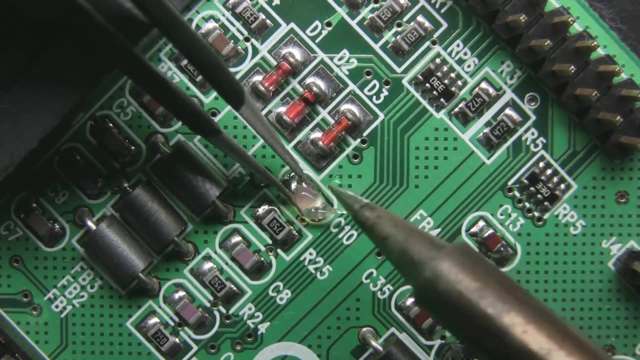 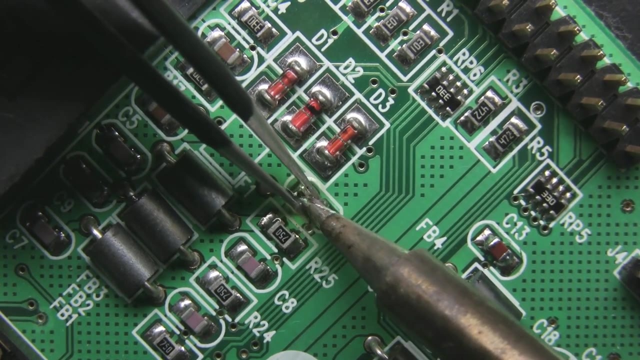 There is a lot of different work involved if you work in a hospital. Fifth is service engineers, also known as customer support engineers. In this role there are two categories: where you fix the machine in your own workshop or either you visit the hospital for fixing the medical equipment. 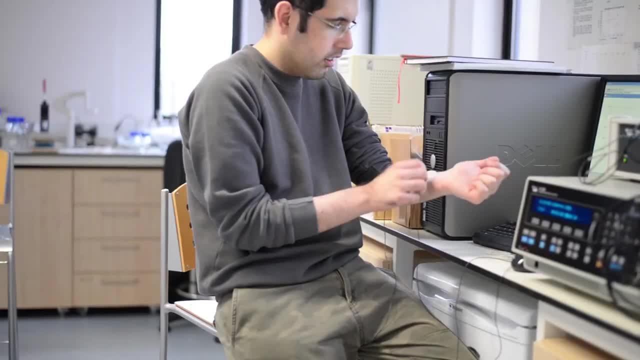